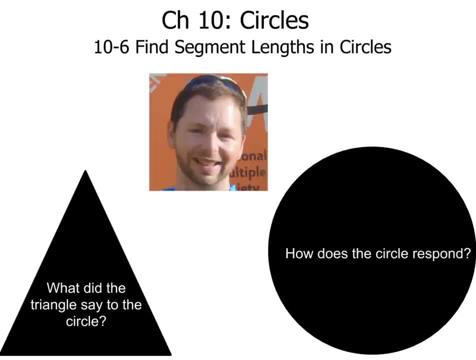 How's everybody doing today? Welcome back for section 10-6 in circles, which is finding segment lengths in circles. Now we're going to have a little conversation here between triangle and circle, And in any conversation a circle is going to give a response. so we'll find out more about that later. 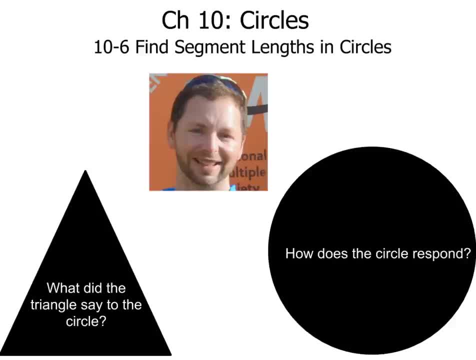 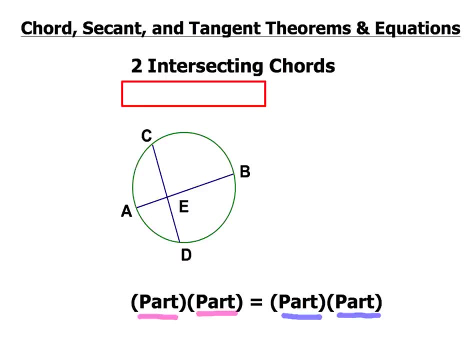 In fact I think there might be a little smackdown going on here between these two shapes, but more on that later. First we'll take a look at some theorems and equations related to chord sequence and tangents. First thing I want to do is take a look at the two intersecting chords. 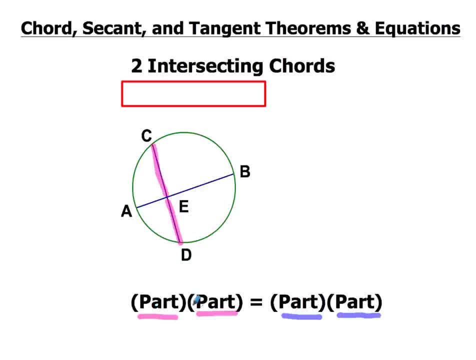 That whole piece is a chord and what I'm going to do is take a look at those two parts, each part of that chord, So from C to E and E to D, and more on that later. And then my other chord is going to be AB and AB. one part of it is going to be from A to E and another part is going to be from E to B. 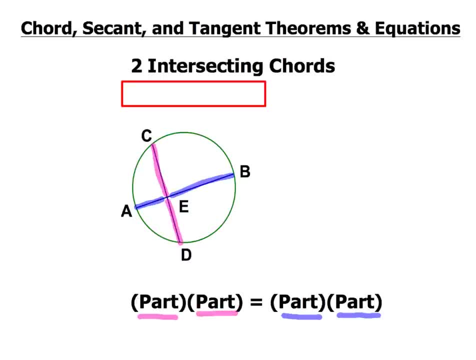 Now, with that said, let's take a look and put those pieces, those words: part times part equals part times part. let's put that into an equation based on that diagram. So here's that equation: EA times EB is going to equal EC times ED. 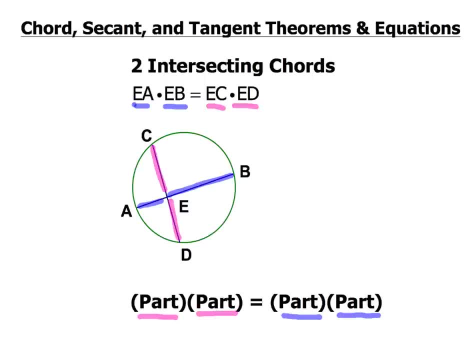 Now, either way you write that, you could write EA or AE either way, but you're taking the parts, the pieces of each one of those chords and splitting them and multiplying them together. Their products are going to be the same. So check this out. 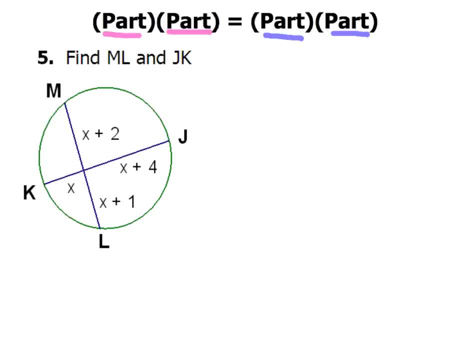 Let's go ahead and get right into an example. Now a little note about this: This starts out with example number five, and that's because it's a continuation from section ten three, which started, which ended with example number four. 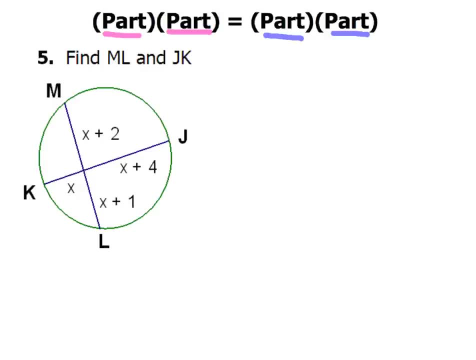 So we're breaking that up into two videos. Here we go. Now. what I want you to do first is highlight the different parts. We've got part times part, so that's one piece right there, and that's one piece right there. 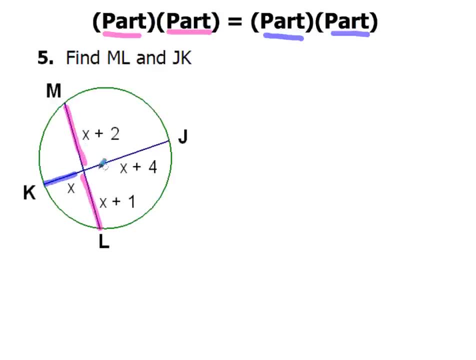 And then my other parts of the other chord chord KJ is going to go from K to that intersection spot and then from there over. So that's going to be. that's going to kind of help me get that set up. 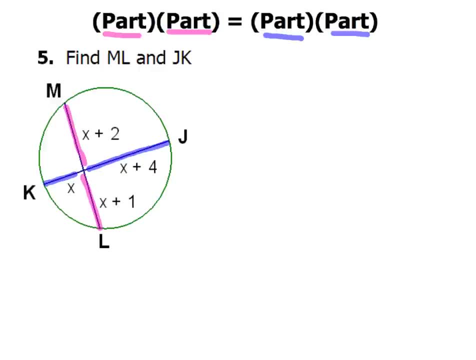 Now we can kind of easily see: part times part equals part times part. Well, one part is going to be this X plus four piece in the X and my other parts of the other chord. that's going to be this X plus two in the X plus one. 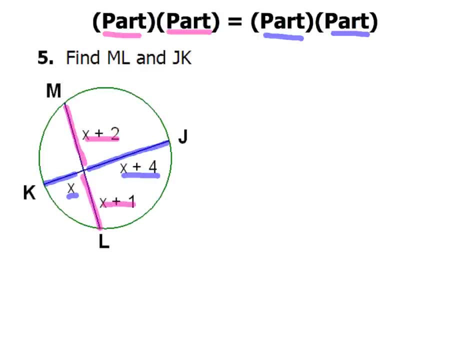 So once I've got all of that figured out, the rest is pretty, pretty, pretty straightforward. So just take your time, do your arithmetic right, So we're going to go ahead and get that set up Now. highlighters help, because then that way you can really see what's going on. 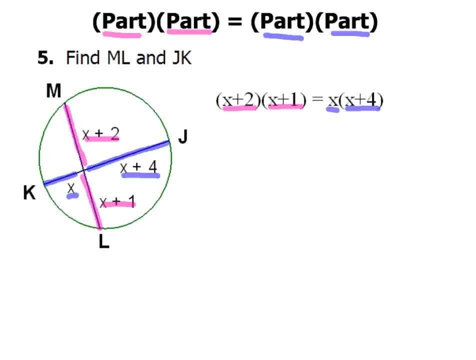 So I have the quantity X plus two times the quantity X plus one equals X times X plus four. So when you do that, just be careful, Make sure that you do your distributive property correctly on that, So we'll end up with X squared plus three, X plus one on the left. 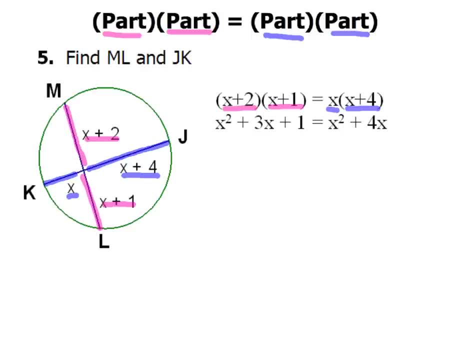 X squared plus four X on the right. Now, if you subtract the X squareds from both sides, right, they are going to cancel out. So when you do that, when they cancel out, you're just going to have three X plus one equals four X. 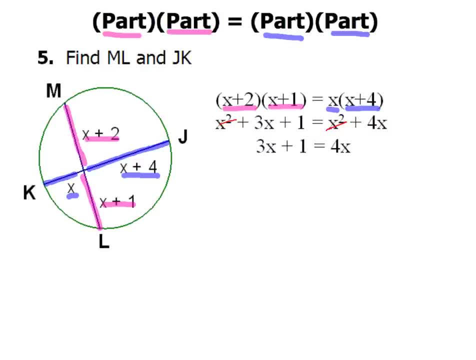 All right, because we're doing this one step at a time. We're showing our work, We're justifying our reasoning And we're just taking our time. Make sure we don't mess up. Don't try and do all this in your head, because that's crazy talk. 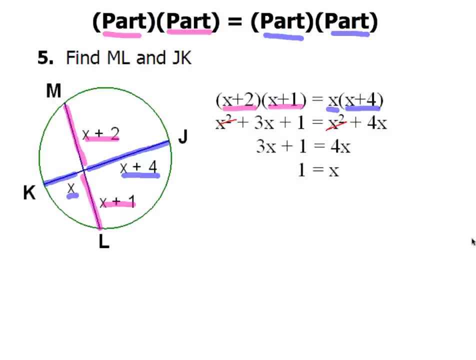 If I subtract three X from both sides, I just get one for the value of X And I'm done right, Sike, You are not done fool. Check this out right here. We said: oh, let's find ML and JK. 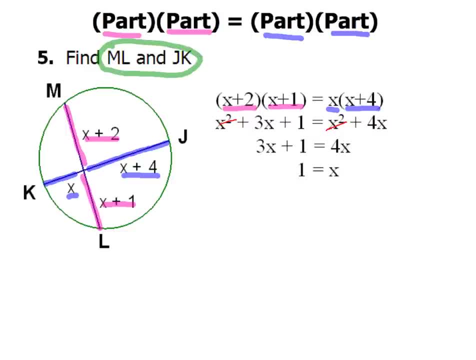 So we've got to take that And we've got to put the value of X Back in to find each one of those values. So take your time and do that And do it correctly, And then see what you got. Hopefully you came up with. ML has a length of five. 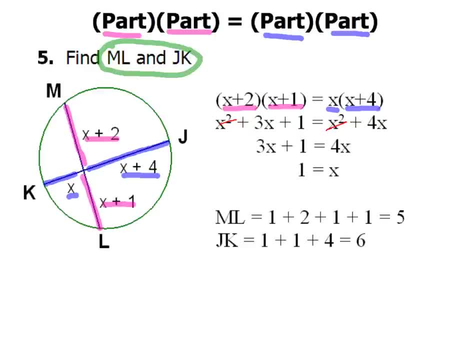 And JK has a length of six. So don't be all foolish and be like: I got X, I'm done. Peace out yo. No, Make sure that you go back and you answer the question. fool, Because a lot of people get us so excited they got X, they forget to go back and answer it. 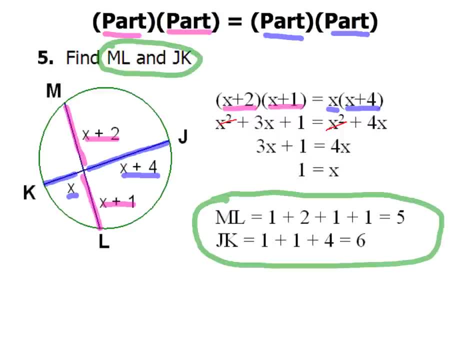 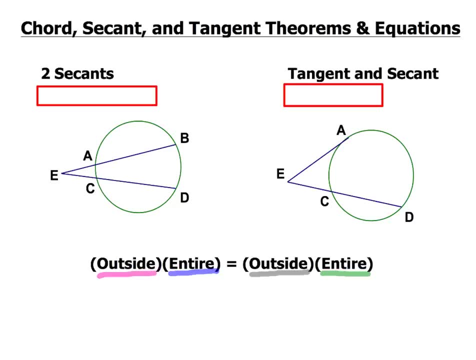 So don't be that guy or that girl. That's one theorem we're going to play with. Now we're going to play with another one. This one's going to look a lot more complex. Check this out Now. this one has to deal with either the secant or the tangent. 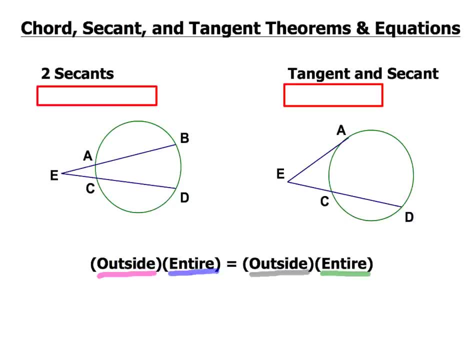 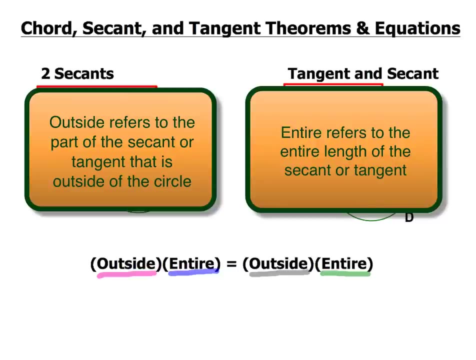 Now we could have two secants, or we could have a tangent and a secant. Now these parts are going to be given two different names. We're going to have an outside and we're going to have entire. So check this out, We're going to do the outside. 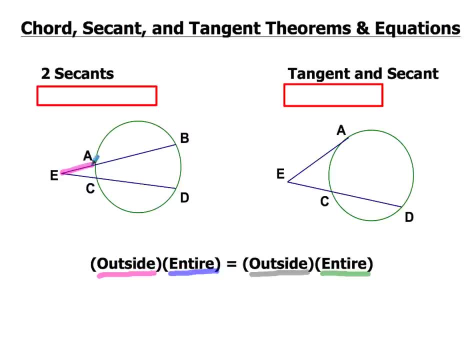 So one of my colors is going to be from E to A And then also over here I'm going to use that same color over here, E to A, because that's both on the outside Now, the entire part of that segment, of each one of those segments I'm going to have from E all the way to B. 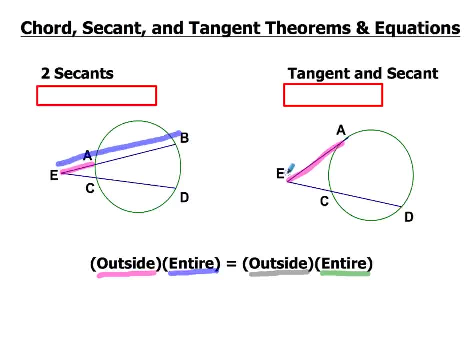 That's going to be that entire. Now, EA, this tangent over here, that segment is going to be the same length right there. So that's one piece, The outside and entire. that's the part on the left side. Now on the right side I'm going to have another outside. 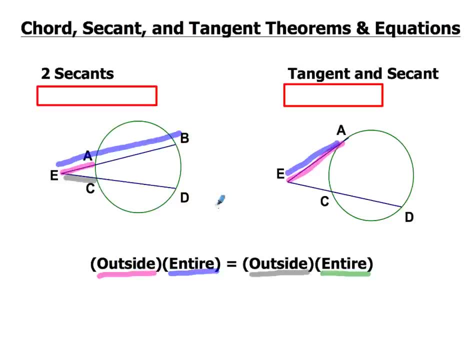 So from E all the way to C, So that piece, and E to C again over on the right hand diagram, And then the entire thing is going to be from E all the way out to D, And then from E all the way out to D again. 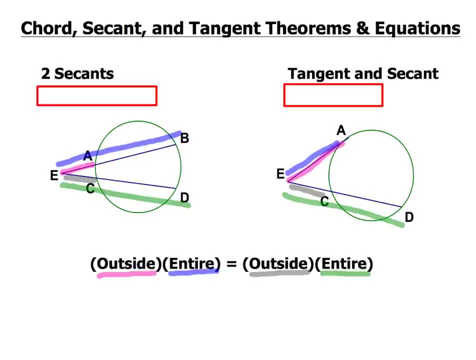 So that's going to be what's kind of going on, picture-wise and word-wise, But we're going to fill in two parts, Two different equations, based on the way we've got those pictures marked. So now, on the left hand side, we're going to have EA times, EB equals EC times, ED. 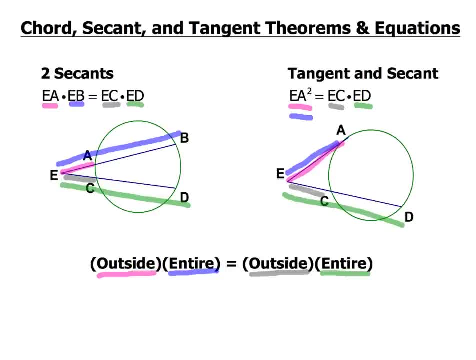 No big deal there. But on the right hand side for our tangent and secant, when we have that kind of intersection going on, check this out: You're going to have EA squared, You're going to have the tangent, whatever that letters are going to represent, or whatever term or variables or whatever. 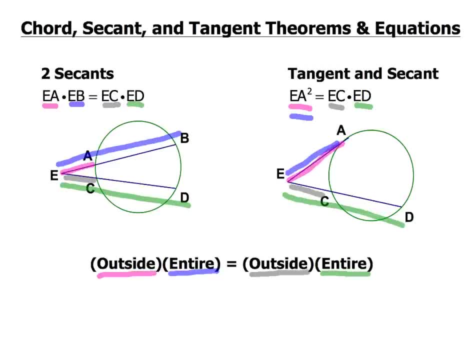 You're going to have that piece squared And then the other part, the secant, same thing. just chop it up. that way, The outside part EC times the entire thing ED. So a lot of people sometimes struggle with that. 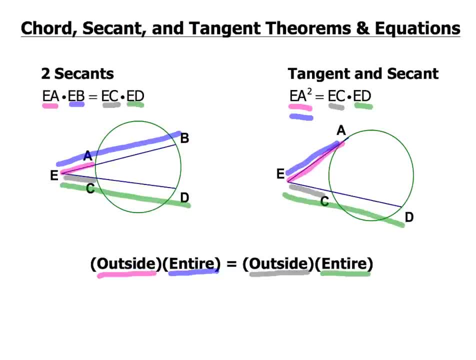 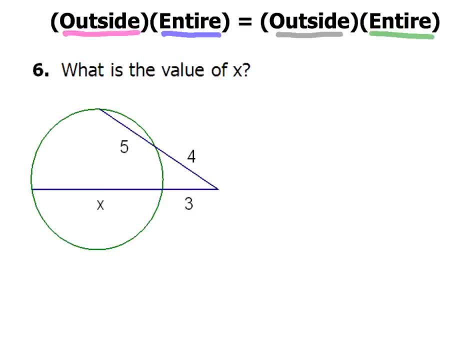 But no big deal. You'll be good because you'll be highlighting everything and rocking through all of this piece. Now let's go ahead and take a look at an example, to kind of play with this. Now we've got outside times entire equals outside times entire. 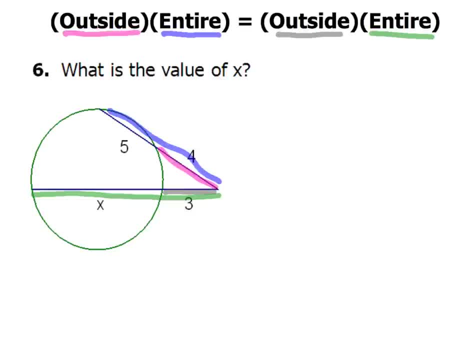 So what I want you to do is go ahead and get everything highlighted the same way I do. So when we fill this out, we'll be looking at the same kind of thing Now, first thing, we're going to take it Now. some people might be able to do the 4 plus 5 part in their head. 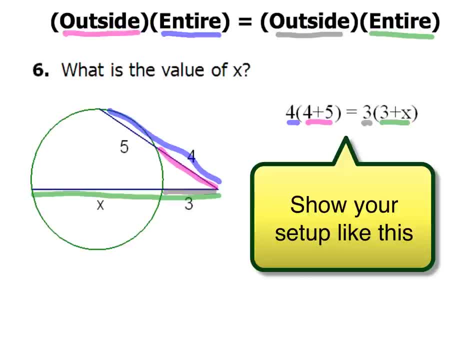 But you're going to have 4 times the quantity 4 plus 5 equals 3 times the quantity 3 plus x, So that's outside and entire for each secant. Now the 4 plus 5, yeah, that gives us 9.. No big deal there. 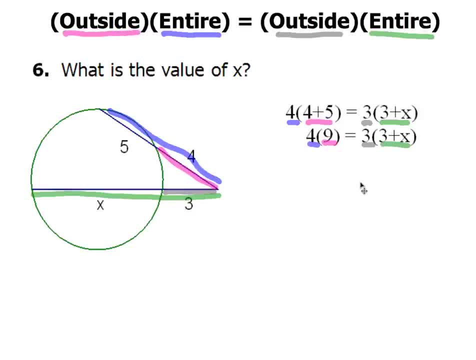 So some people might be able to go right to that step, And that's pretty good. Check this out on the next one, And 4 times 9, 36.. Now, using the distributive property, you end up with 9 plus 3x. 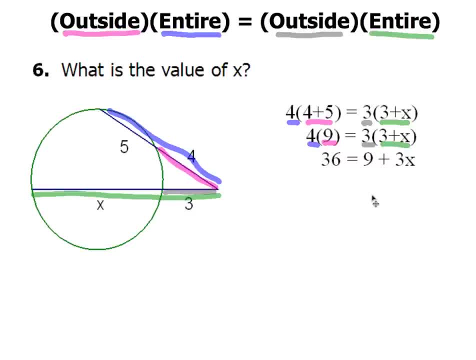 From here, no big deal. Just move that 9 over by subtracting 9 on both sides using your subtraction property of equality, You get 27 equals 3x. Dividing, you end up with 9 equals x. So were we done. 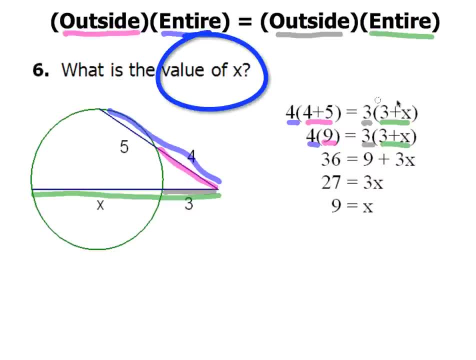 All we were asked to do was find the value of x. The value of x is 9.. So that's it, We're done. Peace out of this question. Not too hard, But again, just take your time. Make sure that you set up your problem correctly. 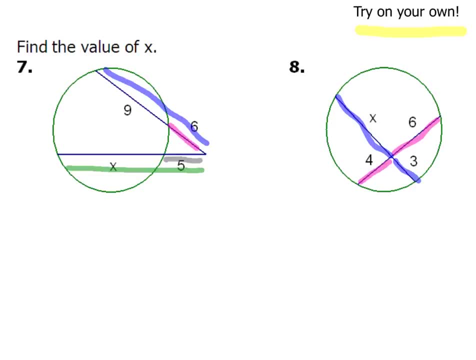 Alright, now, after those two examples, I think you guys are okay. You could probably do these two on your own. Now I'm not going to tell you which formulas to use. You can use those in your notes or what you have written down there. 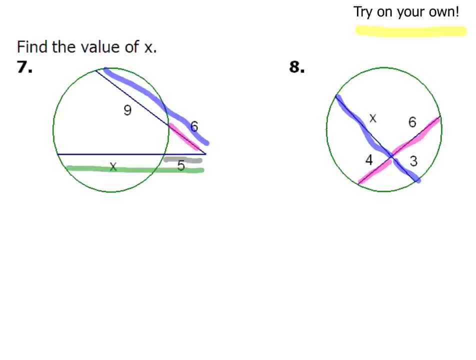 And you can go ahead and get after these Now. I've already highlighted everything. So when we go through and you take a look at the work that I show you guys, it should look like what you have. So go ahead and hit pause. Try these two on your own. 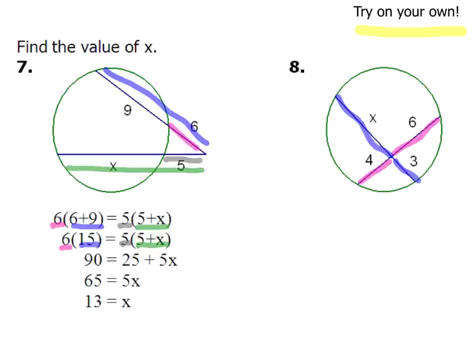 And when you're ready, come on back and check it out. Alright, for number 7, hopefully you came up with a value of 13 for x. Just take your time, Make sure you set everything up correctly and you're good to go. 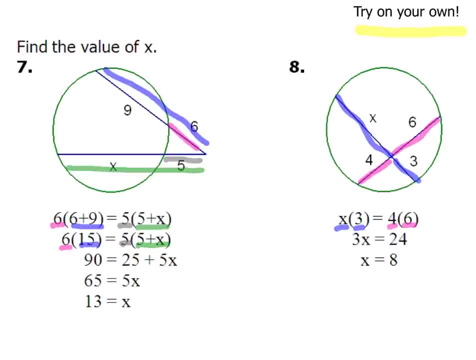 For number 8, you should have ended up with a value of x equals 8.. So there you go. That's how you do those two problems Pretty, pretty, pretty straight forward. Hopefully you got those two correct. Now, on the next one, check out example 9.. 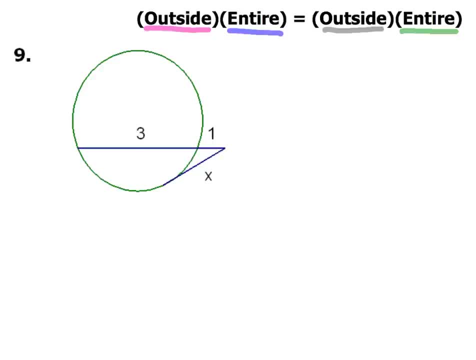 We've got three more examples to do for this one And this one. you guys should probably be okay with it. I'm not too worried about it, But I want you to make sure you go ahead, and this one's going to throw you a little bit of a monkey wrench. 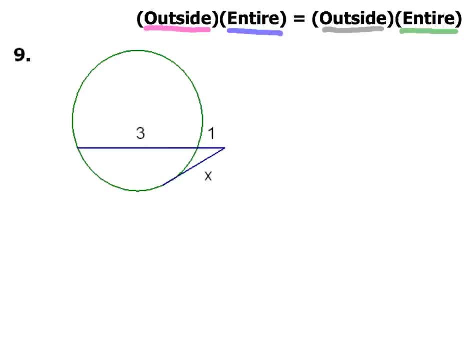 So check this out. We'll kind of go through this piece together. Now, this first part. the outside is going to be this piece right here, And then the entire thing for my tangent is going to be that x again. Alright, so I'm going to have that piece right there. 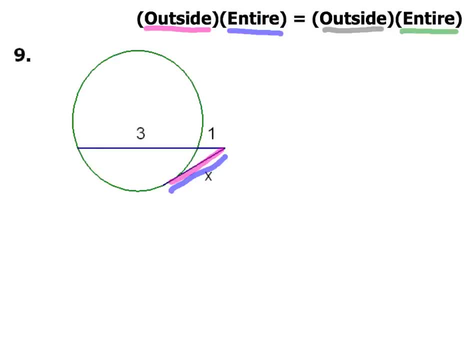 And then the outside of my secant, outside of the secant. well, that's just going to be this 1 right here And the entire thing. we can kind of do that part in our head. We know that entire thing is going to be 4.. 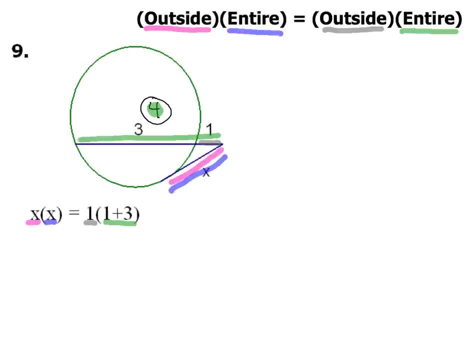 So here would be our setup on this one: No big deal. So when we multiply the x and the y and the x together, that's going to give us x squared And 1 times 1 plus 3, which is just 4,. 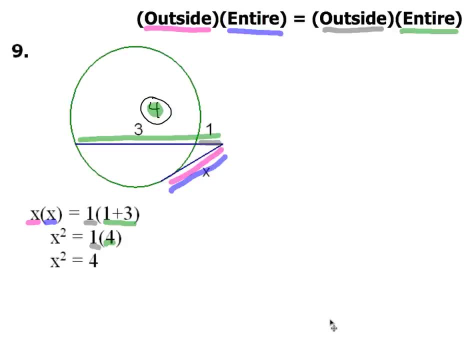 that's going to give us 4.. Now here's where you have to be really, really careful. Most of you guys probably already know this: When you want to solve for x squared, you want to square root both sides. Now don't forget. 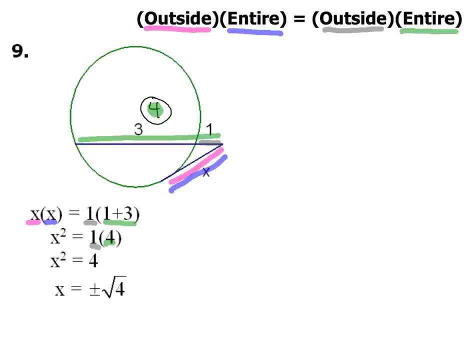 because this is going to come in a lot next year or whenever you take an Algebra 2 course, you're going to have to do the plus or minus the square root of 4.. The square root of 4 is just 2.. 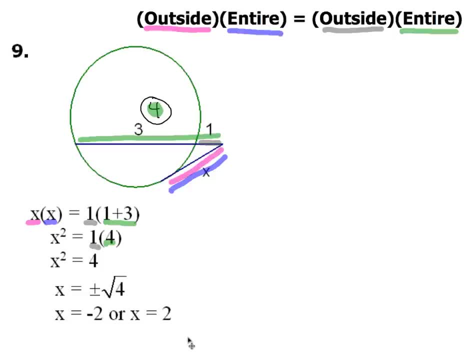 So you're going to have either x equals negative or x equals positive 2, because positive square root or negative square root is a plus or minus. So 1 gives you negative 2 or positive 2.. Now, in geometry, what you have to do, 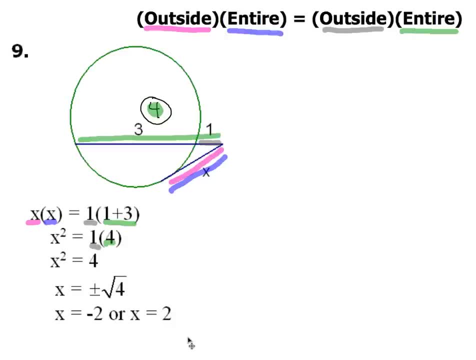 is. take a look at the context of the problem. Where the value of x is, is this tangent piece right up here, So that length can't be negative. So our only solution is going to be: x equals 2.. x equals negative. 2 is what is called a x squared. 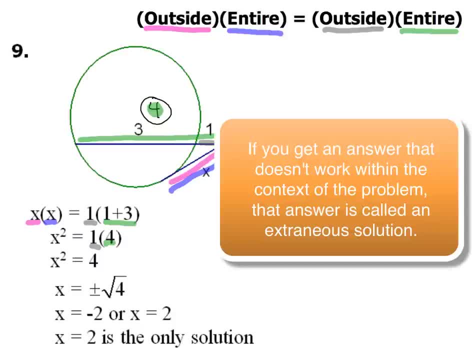 It's called a extraneous solution. So write that word down or say that a couple times to yourself, because you're going to use that a lot in your next level of Algebra course. So an extraneous solution means we get an answer to a problem. 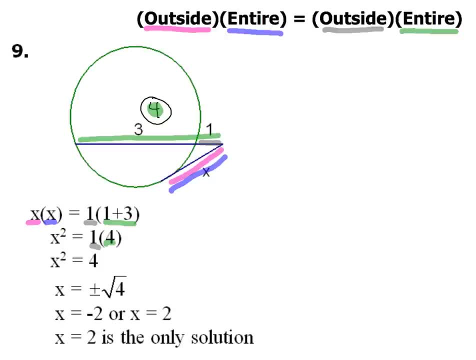 but that answer doesn't fit into the context of the problem, which is what happens here in number 9.. So our only solution is: x equals 2.. Now in example 10,. this one is going to kind of involve the same situation. 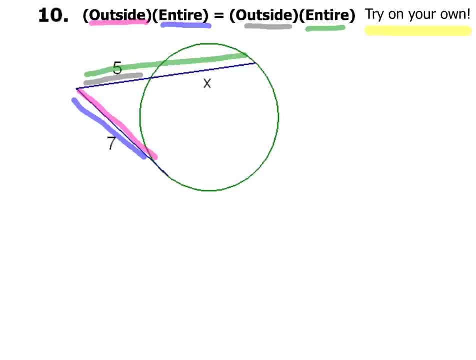 So go ahead and get your highlights on. Take care of doing this one totally on your own. Hopefully you'll come up with the same value of x that I do. Alright, how'd you do on this one? Hopefully you came up with 4.8 for the value of x in your work. 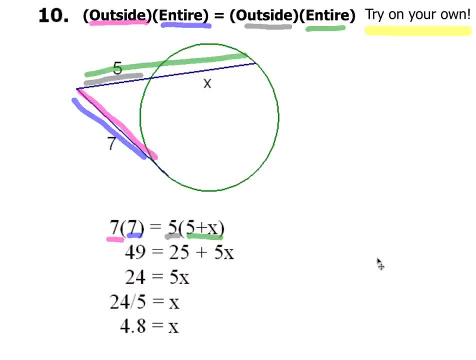 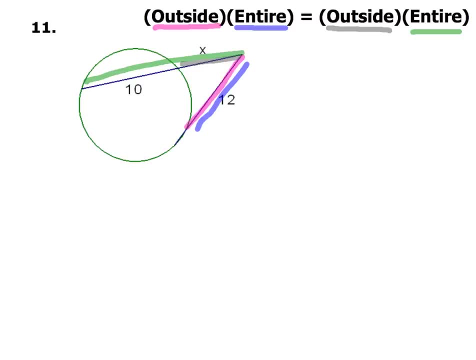 It's just as nice and neat and organized as it's shown right here. So make sure you take your time, Do your arithmetic correctly. Boom, you got it. No big deal, Alright. so you guys have hung in. Here we go with our last example. 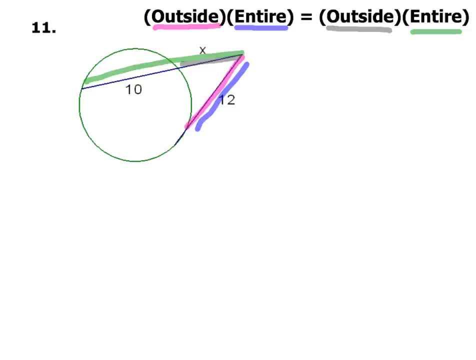 example number 11.. We're going to go through and do this one together. Same kind of stuff as before. Outside times entire, equals outside times entire, No big deal. But we're going to run into something a little different here. Check it out. 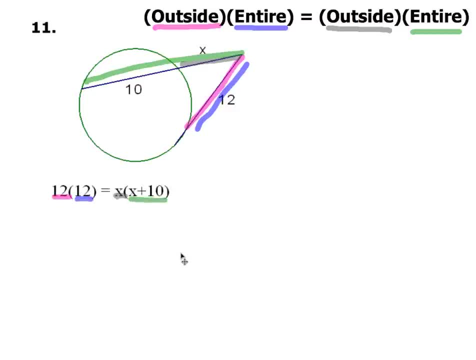 We'll set up our equation. No big deal. I think you guys will be rock solid on that piece. But when we distribute this time we end up with 144 equals x squared plus 10x. So with this type of problem, 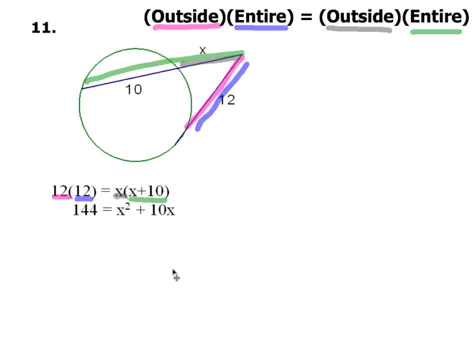 what you want to do is get, when you have a squared on one side, you want to get the other side set equal to 0. So what that means is we're going to subtract 144 from both sides. When you do that. 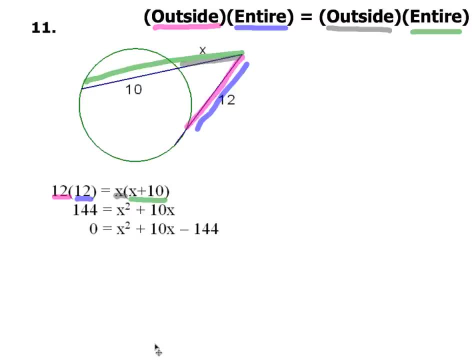 you'll end up with 0 on the left and then x squared plus 10x minus 144 on the right hand side. Now, from here you're going to have to factor the right hand side, So I need two numbers that multiply together. 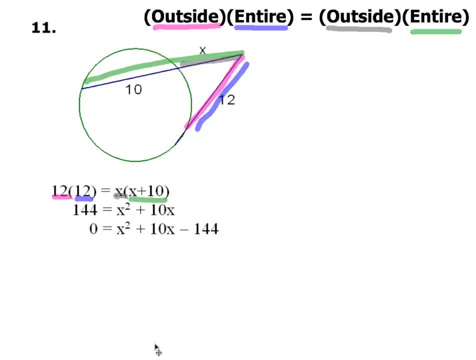 to give me negative 144, but have a sum of 10.. You play around with that for a little bit. Use whatever skills or mad math stuff that you got going on And you'll figure it out. When you do you'll get one factor is going to be x plus 18,. 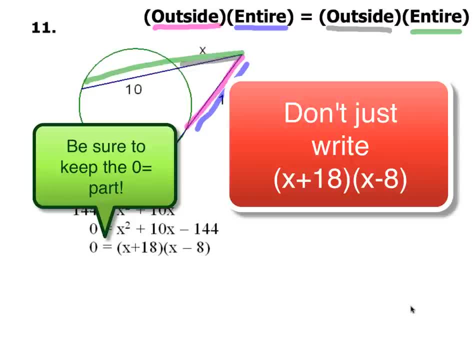 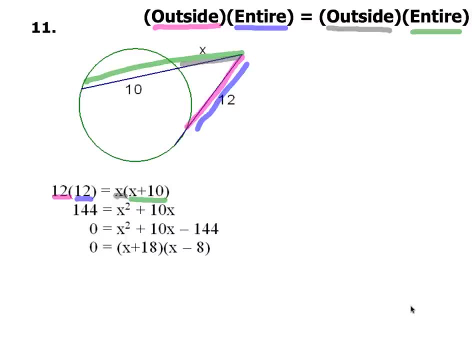 and the other factor is going to be x minus 8.. Now if you were to use the distributive property twice- or a lot of teachers will call that FOIL- with x plus 18 times quantity x minus 8, you'd end up with a previous step.